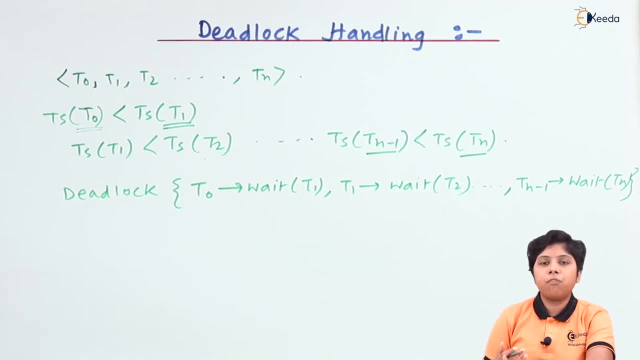 Now there are three ways for this deadlock handling. The first one is prevent from a deadlock. that means we will arrive in such a condition that the system will never enter a deadlock and we are ensuring that. So that is the form of deadlock prevention. 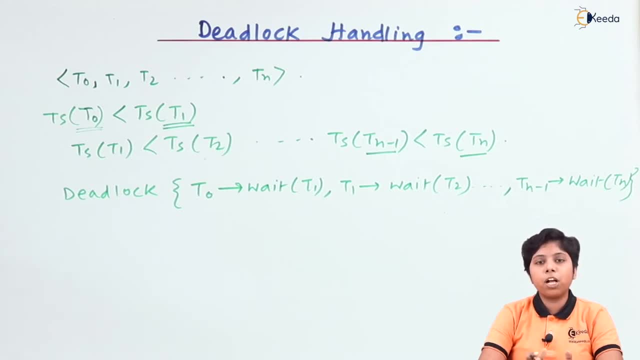 The next one is deadlock avoidance. It means we will avoid in such condition that will happen for a deadlock And that cannot be done. Kawashima, please let me have another deadlock. So the similarity between prevention and avoidance is for prevention. we are not. 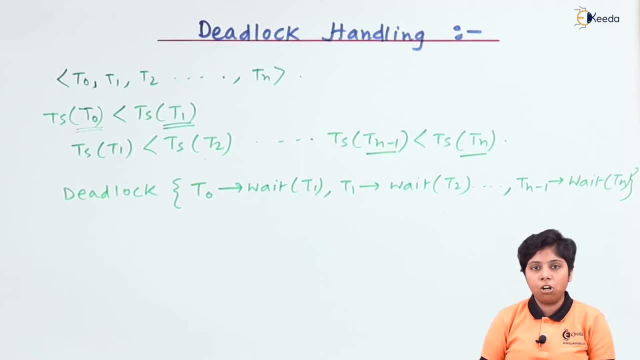 considering the conditions that can arise with the deadlock and for avoidance. we are conditioning on this particular predicates but not allow them to be happen, to arrive in a deadlock. And the final one is the deadlock avoidance or the deadlock recovery. that means the deadlock has been already occurred and we need to recover from that deadlock. So the rolling back of 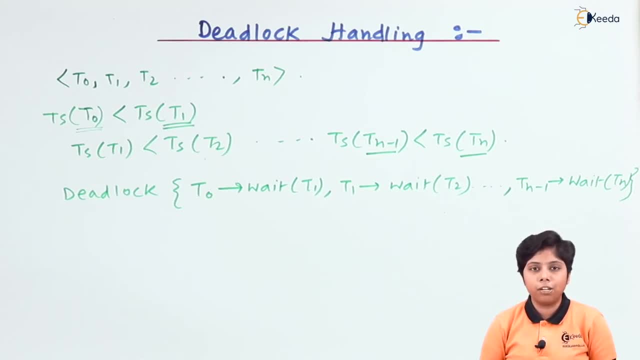 transaction is a way of both the prevention and deadlock recovery, but into different situation. So first we will talk about the deadlock prevention. The first approach for deadlock prevention is no cyclic wait. that means here we are having a cyclic wait in this deadlock state. So if we can confirm that there is no cyclic wait of the transaction for another transaction, 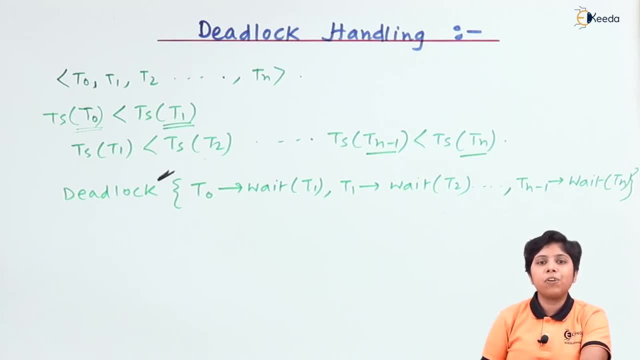 that is in time stamp, credit to it so we can avoid or prevent the deadlock. The another is more closer to the deadlock recovery. that is, other than waiting, we are using rollbacking the transaction to a state that the transaction will now cannot enter this deadlock state. 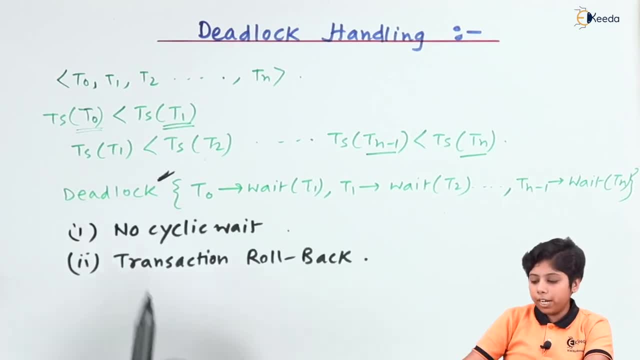 So the first one is now the first one we can achieve by locking this data item. now, when we provide that lock on a particular data, then we can ensure that the read or write operation can be performed only by acquiring an appropriate lock on that data item. so now we can have the particular lock on that data and then 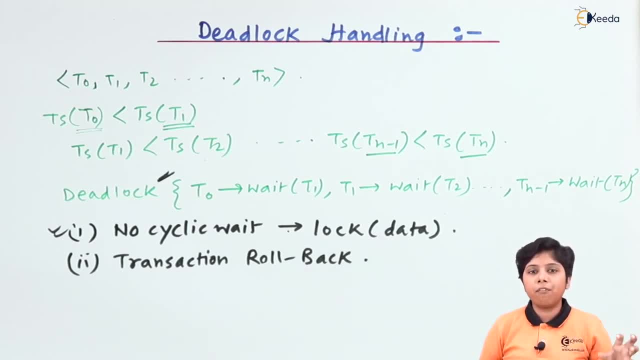 can perform this waiting. so now we will never wait for such a condition that if the lock is not occurred, we will not wait for the data to perform that particular operation. so we will never reach this no cyclic weight condition. and the second one is transaction rollback. see, there is when. 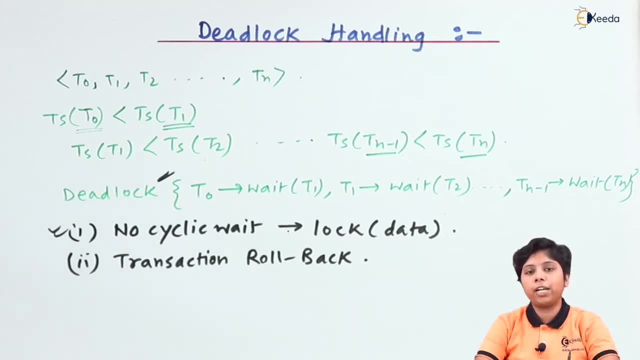 we are waiting for a data item other than having the lock on that item. so now we can roll back the data item if there are two more timestamp that is greater than the timestamp of this transaction ti, so we will arrive this transaction roll back to avoid this deadlock. so now, when we are 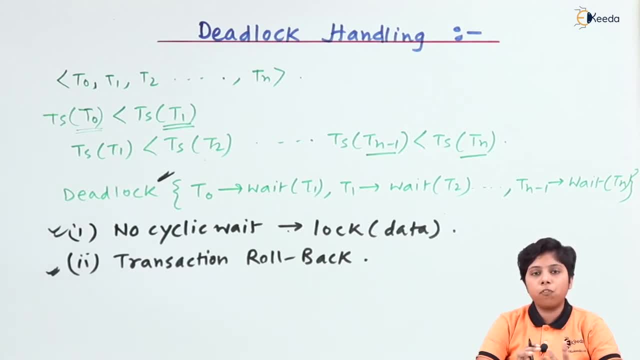 talking about this: no cyclic weights. there are two types of ordering. first and last is the non-cyclic weight, so this is the one where the transaction rollback will take first. one is the ordering of all data items. when we have this ordering of all data items, then we can say that every data item that we are considering must arrive in an order so that we 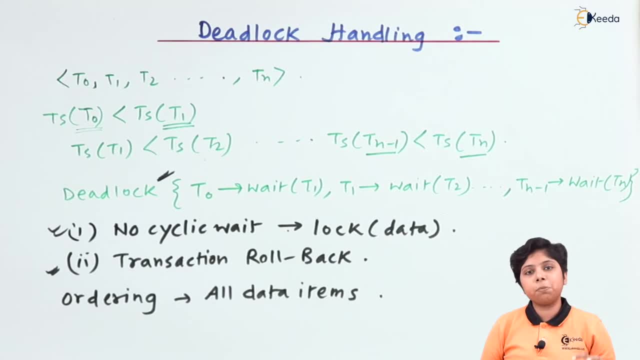 will not enter the deadlock now. my data items will arrive that first. if transaction ti is performing and read item on this queue, then we cannot have that queue to acquire a lock that is acquired by an exclusive mode on another transaction. so in this way we must define an order so that we are 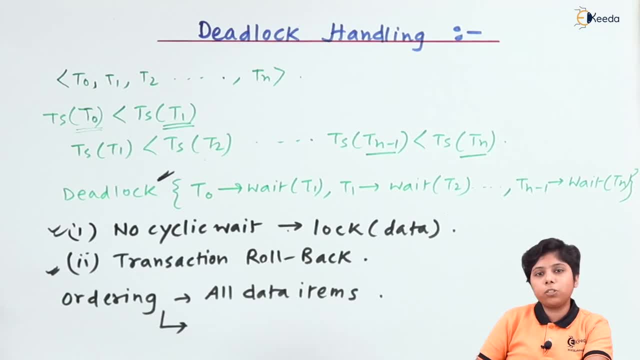 having all data items ordering. next one is an total order of data items. the total order of data items suggest for that we are having in such a way that if an data item has an exclusive lock that is acquired by a transaction ti, that we cannot have that item or the request for a lock. 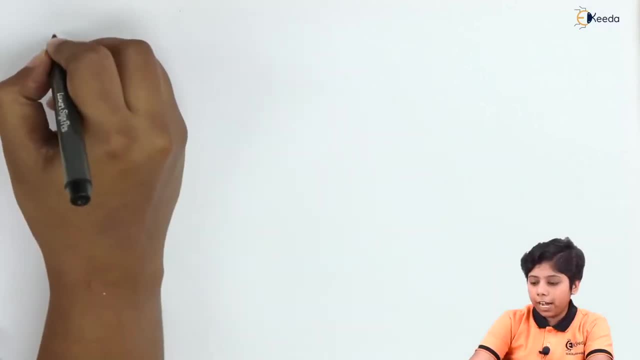 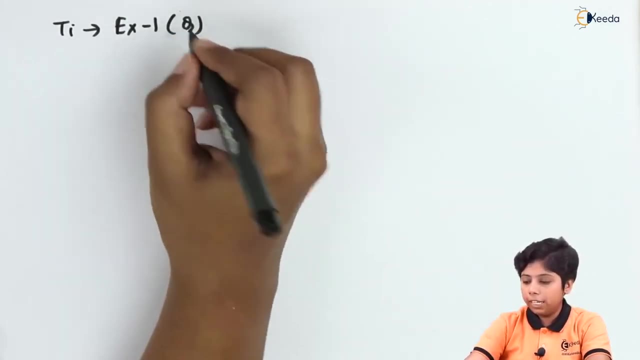 if it is proceeding on a transaction. so now, before the order wordt under low code's order, it should not be in the order code. so if data items, if ti is given an exclusive lock on a data item, q, then if the ordering is already based q, r, s, t. 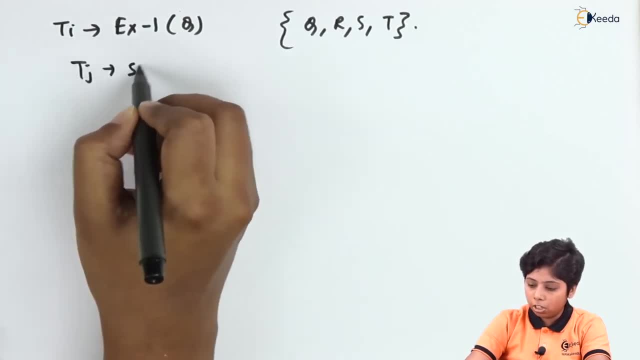 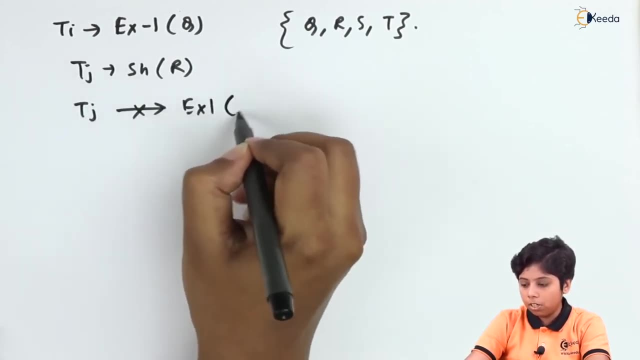 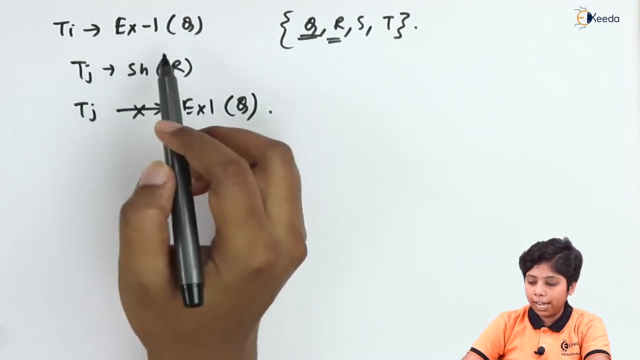 so now if the tj is acquiring and shared lock on data item r, so tj cannot perform to have and request on an exclusive lock on data item q, because q belongs to proceedings of r and no transactions can have the item that has been preceding in another transaction. 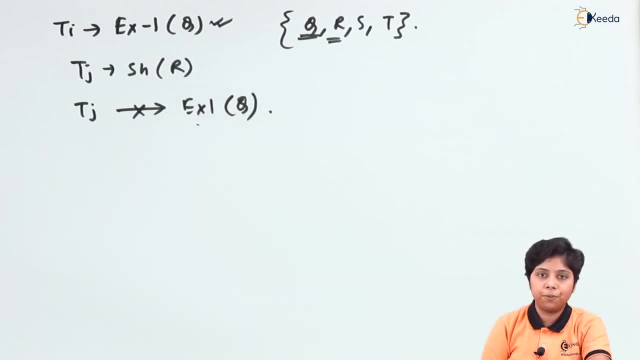 and produce an exclusive lock in that transaction. so in that way the total ordering of data items can be ensured with the conjunction of two-phase locking protocol, that we are having an exclusive lock on the data item first and if there is a net then we can have the shared lock. 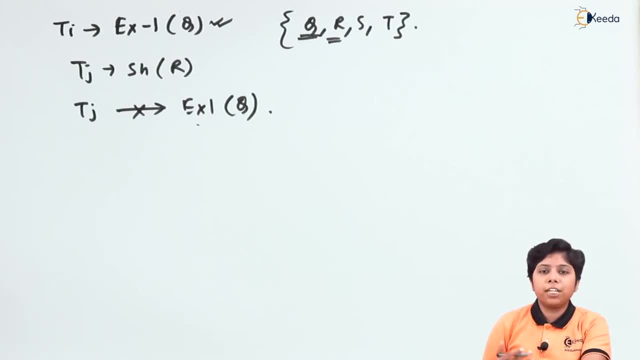 but not the vice versa. and now we will talk about the transaction rollback. now the second approach of this transaction rollback implants are this: preemption of data items. that means, if a transaction is already performing, then on best, some conditions, we can preempt the transaction with another transaction to avoid the deadlock. and in that way we first need to roll back the 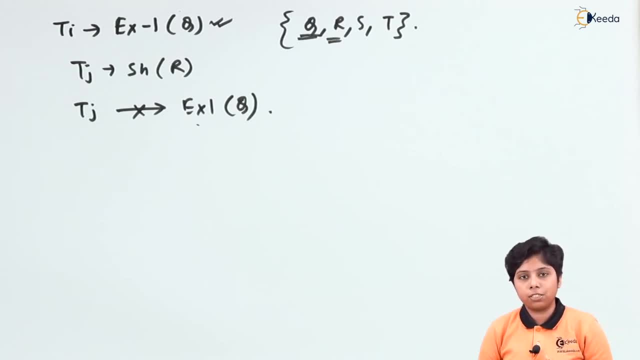 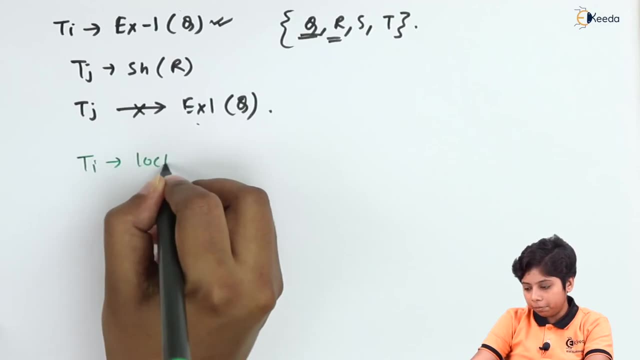 first transaction and then we can preempt the second transactions. so let us define this with a second transaction and then we can preempt the second transactions. so let us define this with a denotation: if ti has log granted on a data, item q. now if tsti is greater than tstj, that means the 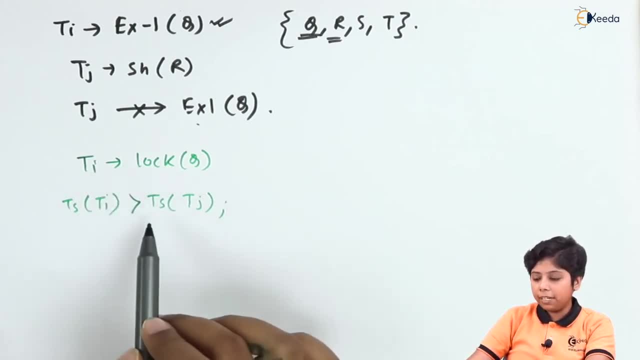 data item that is arriving before ti and but ti is having this lock on this data item q, then tj will preempt and have unlock on data item q rather than ti. what is having? so tj is being preempt- that particular ti to have performed its locking on that particular data item q. now the preemption. 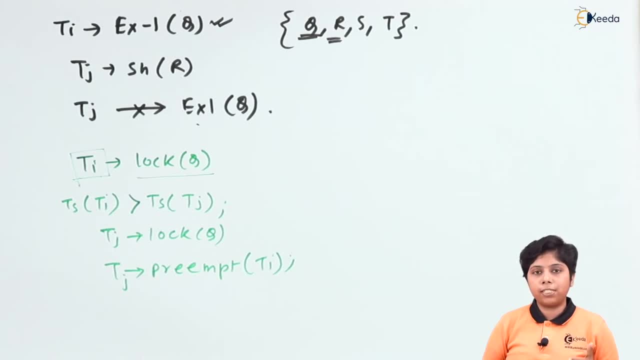 and the rollback will go for these two algorithms. one is the wet die, another in this vent and recover. the vector algorithm supports for no preemption that if there is also the tsti is greater than tstj and ti has acquired a lock. so tj needs to wait until an unlit ti releases the lock. 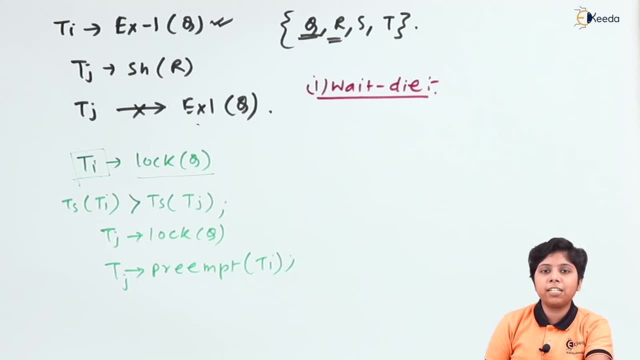 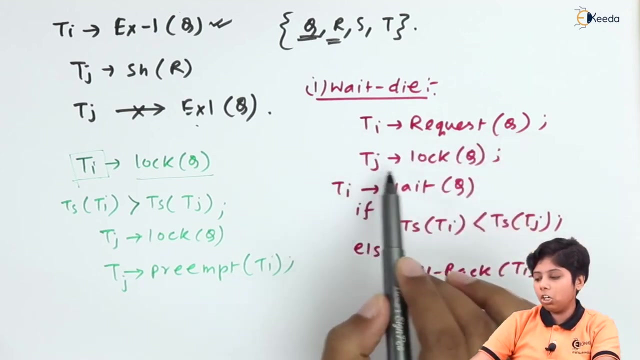 and has performed its operation. now it believes that ti will perform its operation on this data item q very nearly and tj can perform after that execution of ti. now say, if ti requests foreign data item q which is acquired and locked by transaction tj, now ti is allowed to wet only if 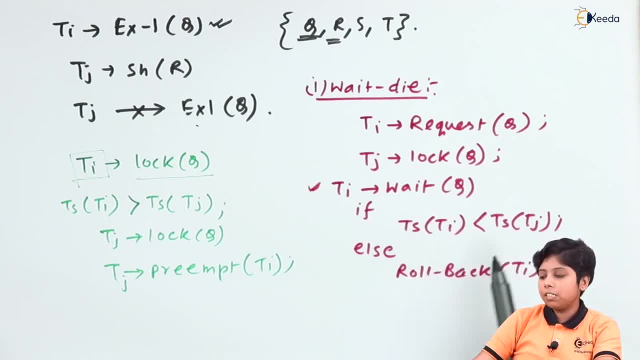 tsti is less than tstj, that means the ti is preceding the transaction tj in the schedule s. otherwise we will roll back ti because we were killing it and ti was no wet. because the ti will not perform, the tj will happen next and then have the lock. so now when the tj, which will happen after the ti has, 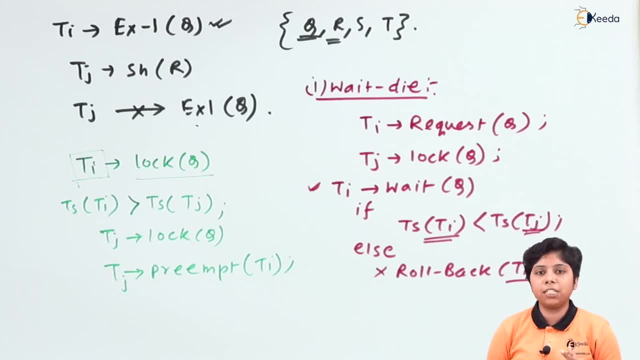 acquired the lock, how ti can perform? it will enter the deadlock if there is no wet die algorithm followed by it. now let us suppose t1, t2, t3, three transaction have is 5, 10 and t15 times time respectively. so now we have tn with 5, t2 with 10 and t3 with 15.. now if t1 is requesting a lock, 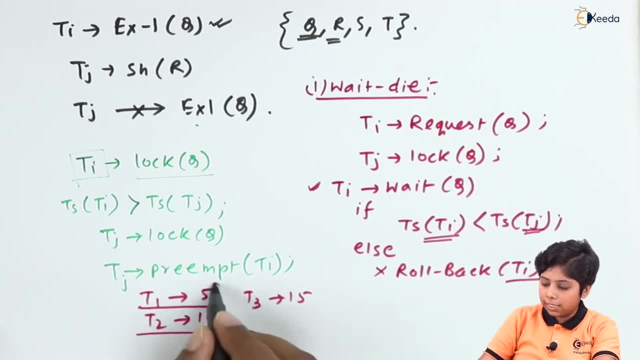 that is, t2 is acquiring, so 5 is less than 10. that is followed by this one, so t1 will wet. that means t1 will go for this weight on t2. but if t3 is requesting something that t2 is holding but t3 is happening greater than 10, that is, 15 is greater than 10, so it will roll back this ti. that. 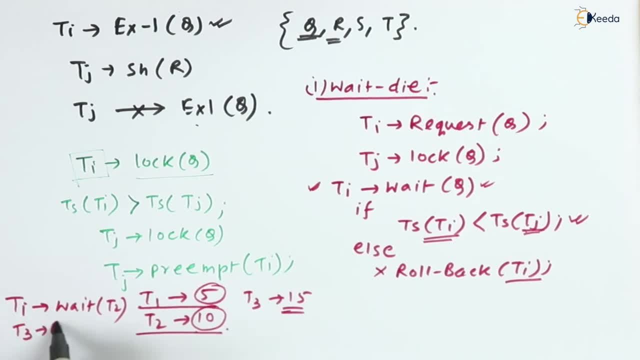 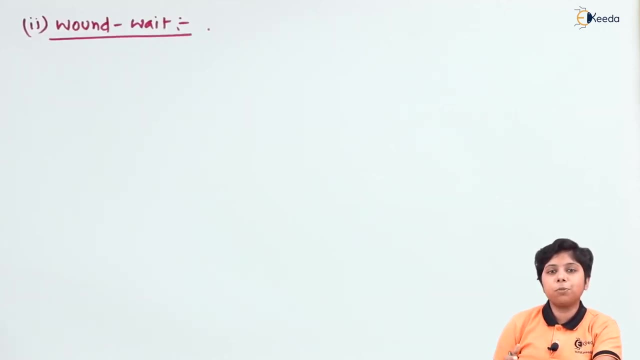 means t3 will be roll back. so in this way we can suggest that the weight and roll back, that is a weight die algorithm, followed by within this time step ordering. now let us go for this next algorithm. now the wound wet is in counterpart of this weight die algorithm, so now we are having that particular 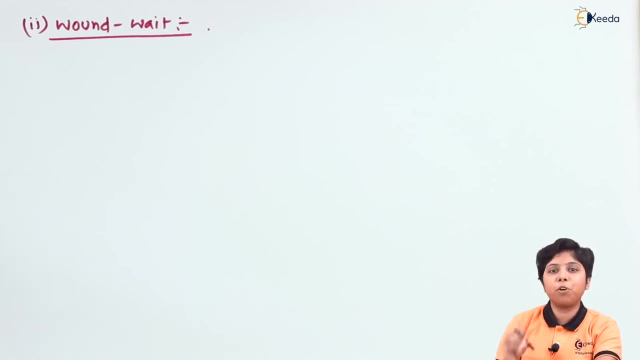 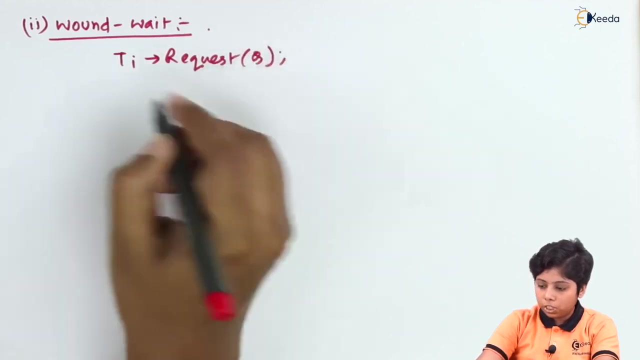 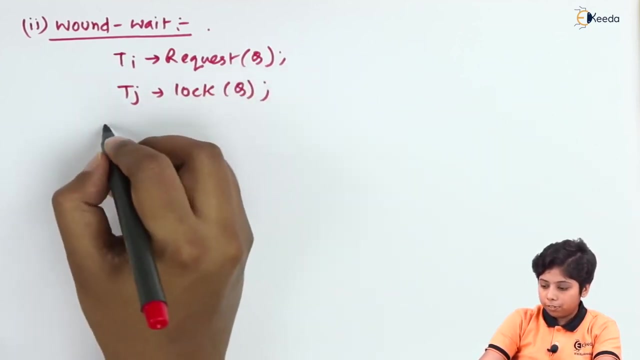 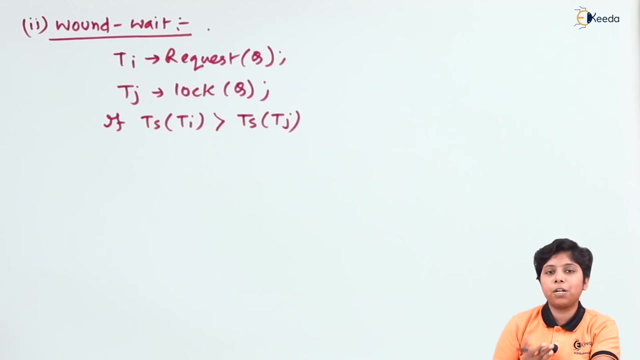 493.07.309, but is younger than Observe warning of a test for 100. Now we are actually reversing the counterpart of this wait die algorithm. TSTI is greater than TSTJ means TSTI is younger, So if it has got a greater timestamp, that means it is the newer one to editor. 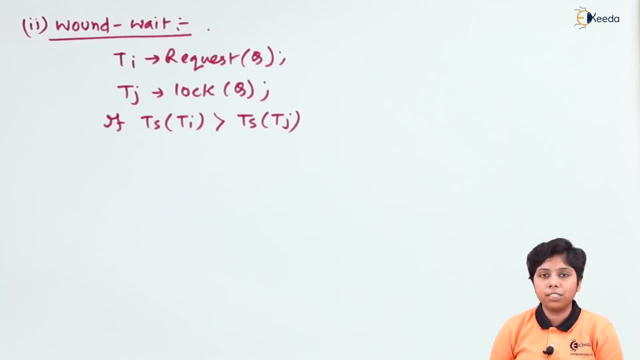 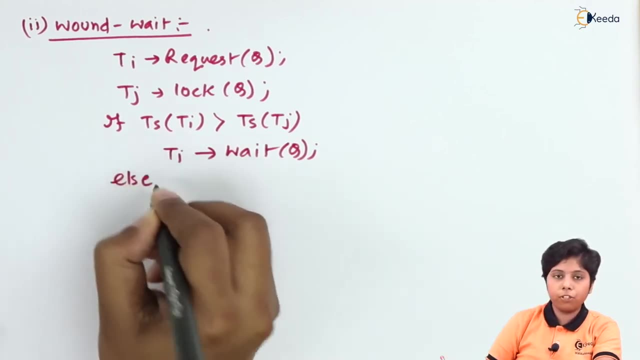 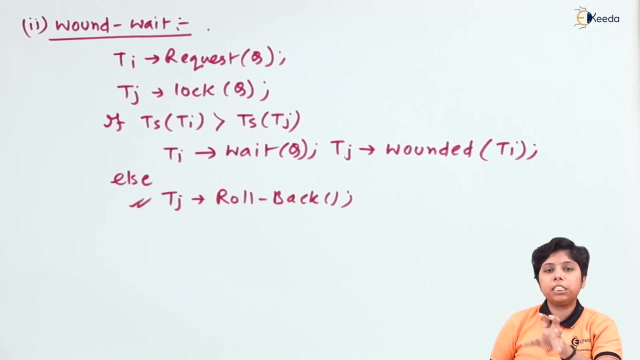 So now TI can preempt the data and can wait for this queue. So now my TJ is being wounded by TI, So else we will wind up this TJ, Otherwise we will roll back this TJ, While roll back TJ means we are having the TJ being preempted by TI. 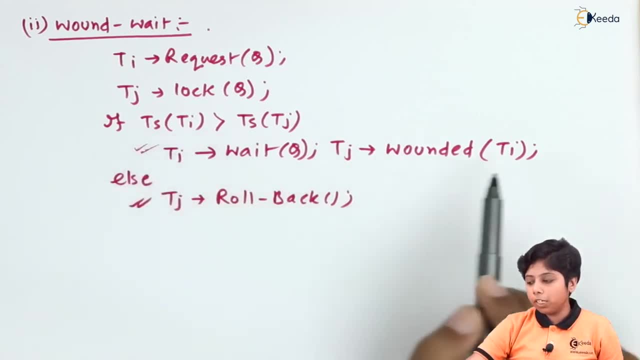 Other than TI will wait. So now it is being wounded by TI or it is roll back by TJ. So what we are having other than roll backing the item or the transaction that is the new one to enter, We are roll backing the item that has been executing as a preemption to the new item. 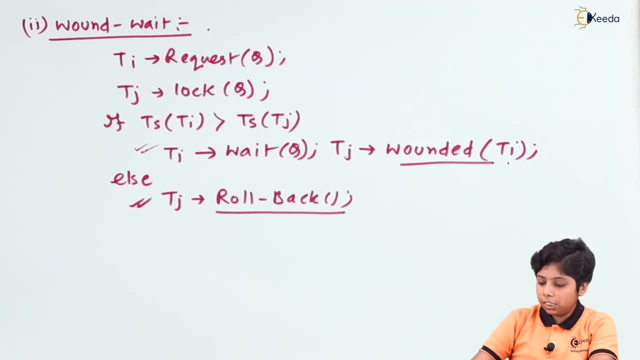 So now, if we take example of the previous one, that is T1.. 5, T2, 10, T3, 15.. So now, if T1 is holding an item and T2 is waiting for that or requesting for that item, 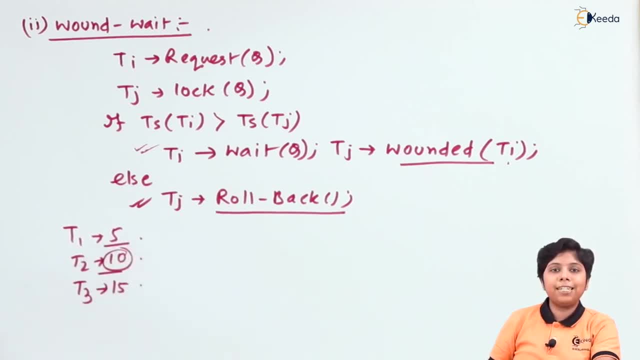 So T2 is greater than 5, that means it is newer one. So T2 will wait. Now if T3 is happening on T2, that means T2 has acquired on the lock or T1 has acquired on the lock And T3 being this requesting one. 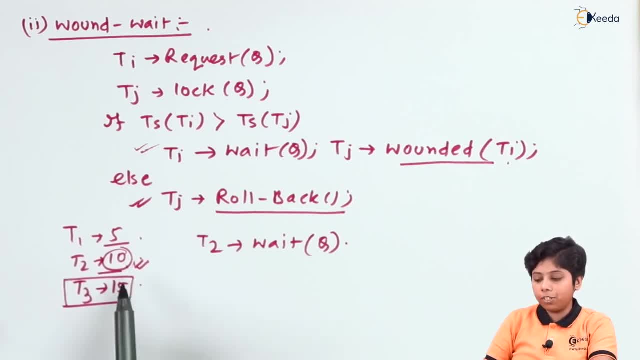 So if T3 is a requesting one, then we can say that 15 is greater than 10.. Then also T3 will be wait for Q. Now what happens when T2 is the lock that we are having and T1 has requested for a lock? 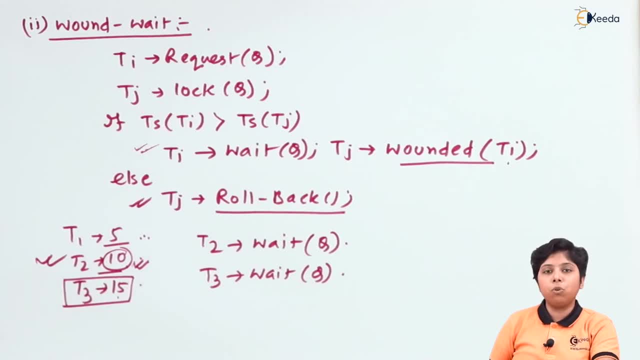 And T1 is greater than on this Q. That means T1 has a larger timestamp than this T2.. So what will happen then? T1 will be preempted And T2 will be rollback. So in this way, the wound wet algorithms is also a counterpart for the wet die algorithm. 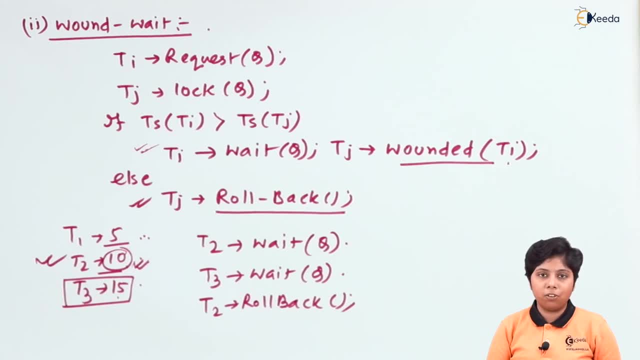 And they both stands for the prevention of this deadlock. Now, the problem with this technique for prevention is this unnecessary rolling back. Now, whenever we are having this rollback, sometimes it is not mandatory or necessary to have that. So to avoid this expensive rollbacks, we can have the similar techniques with this lock timeout. 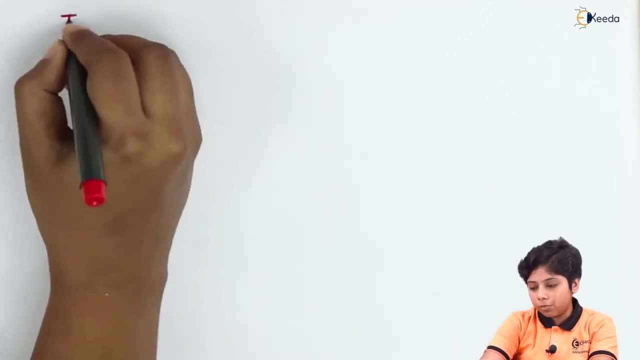 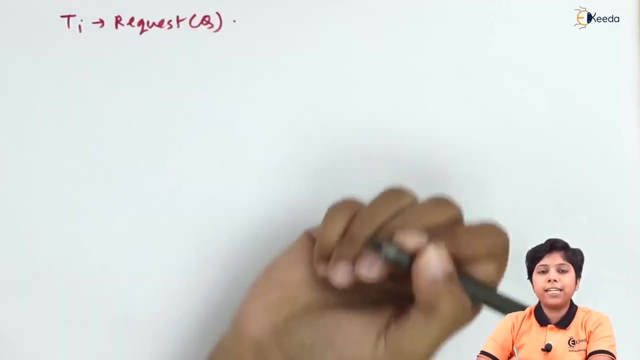 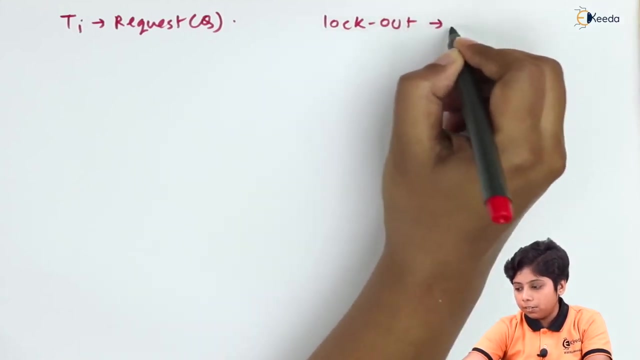 So we can have the same mechanism Now in this lock timeout. say, if T1 has requested for a particular data, item Q, Now we are setting a lock timeout value or the lockout value. See the lockout value is 7.. Now T1 is acquiring the lock. 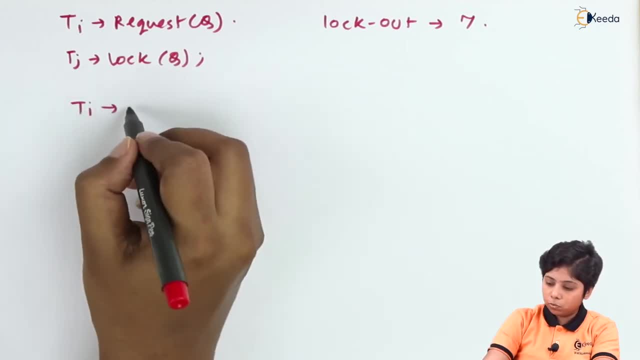 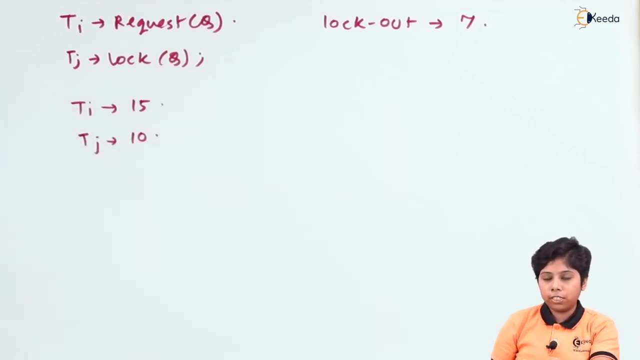 So T1 is having 15 and T1 is having 10.. So T1 is the newer one to enter and T1 is 10. So that lockout time of T1 is 7.. So there is no preemption. 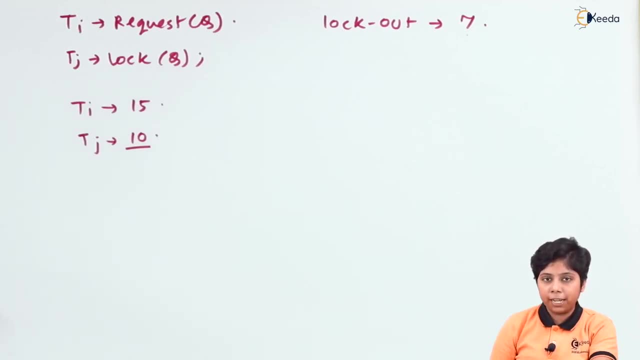 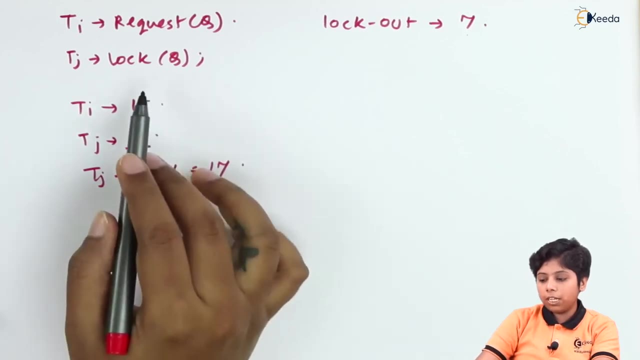 There is particular locking out on that particular time. So now T1 will acquire the lock till 10 plus 7 at 17 seconds. So now T1 waits for 15 and enters the system at 15.. So the locking out is 17.. 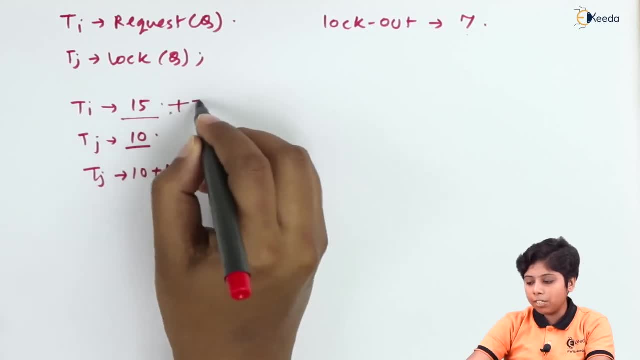 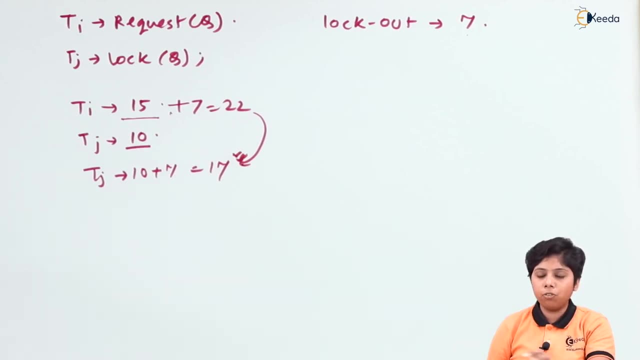 So it waits. So it waits for 7 seconds. That means 15 plus 7,, 22.. So it's 22 is greater than 17.. So the locking timeout is greater than the lock value. So now the lock timeout is greater than the lock value for this particular transaction, T1 and T1. 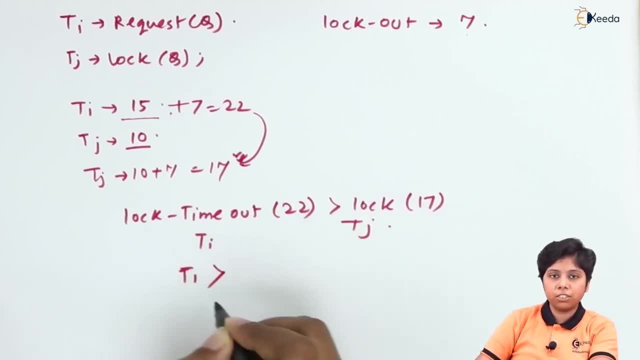 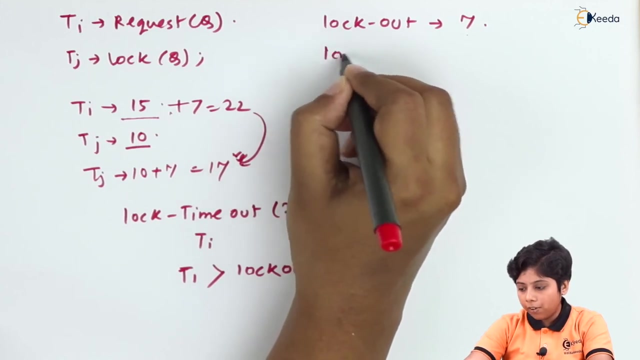 So now T1 will be performed onto this lock. Now again we have that, this T1. And waits for a second. that will reenter the value. That means, say, suppose the lockout is 7 and the lock value is for 14 seconds. 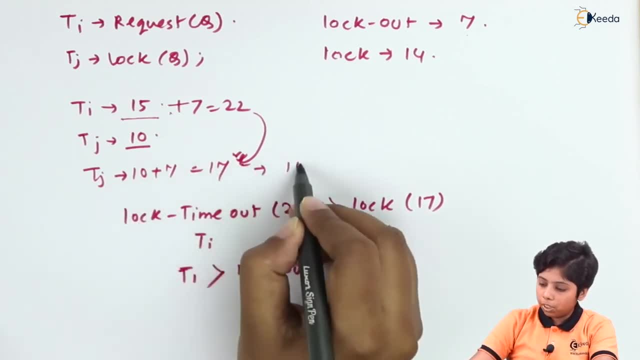 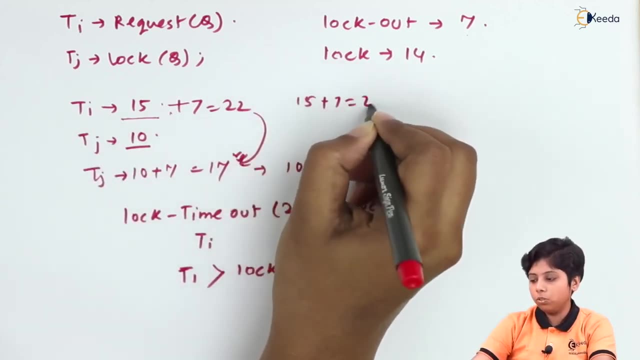 So now it will have 10 plus 14, that is 24, and the TI will have to wait for 15 plus 7, that is 22.. So after 22 it cannot just stay back. It will restart itself and roll back itself only. 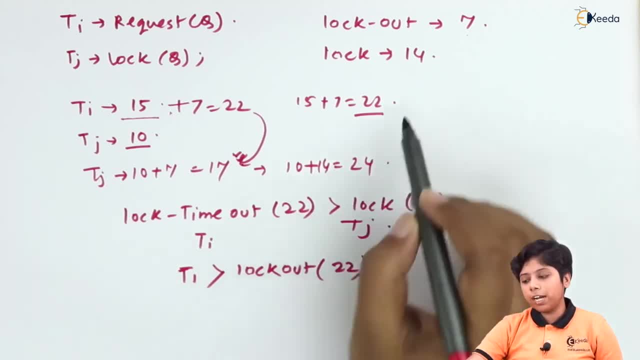 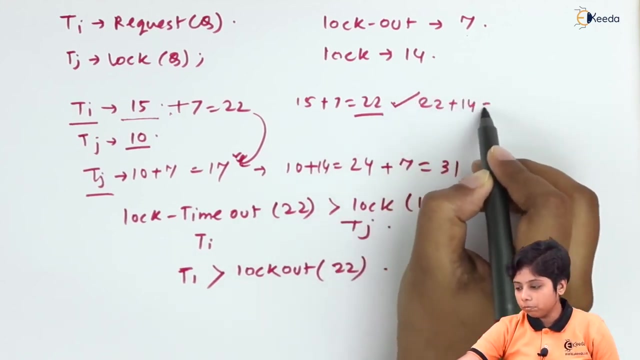 So there is no force rollbacking. It waits for a time, a counter period of, and after that it will roll back and restart yourself, Because by the time it believes that next time when TI will arrive, TJ will be finished its task. So now, 14, 24 plus 7, that is 31, and it will have this 22 plus 14, 36.. 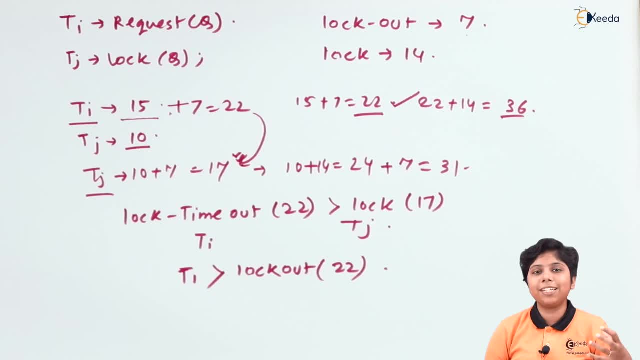 So now 36 is greater than 21.. So now TI can enter the state because that time TJ is supposed to be finishing its task. So in this way, lock time out is an another approach other than avoiding this unnecessary rollbacks for this wait-tie and one wait algorithm for the deadlock prevention. 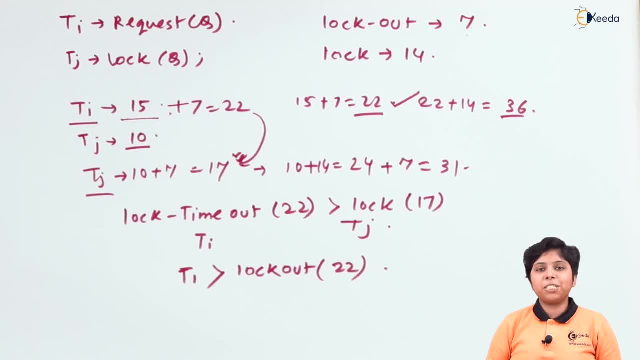 This transaction on this lock time is out algorithm is particularly easy to implement But, However, we will say that particular transaction will wait for how much time, that the lockout will be performed on a day and a half Or, for those who are familiar with this process, lock timeout will be based on which things? we do not know that how much time it will be taken for locking a particular transaction, so then it will again can lead to a deadlock by waiting for a long time for that transaction. so that is why in some systems it is avoided for this lock timeout. 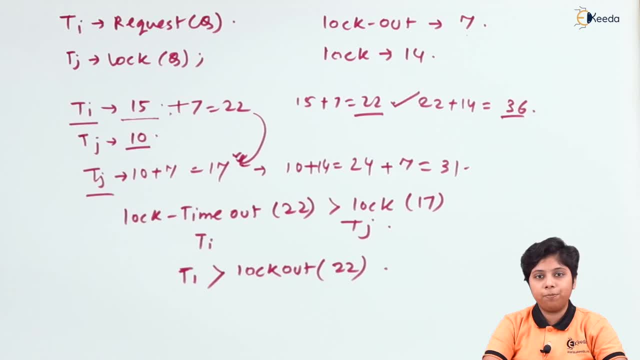 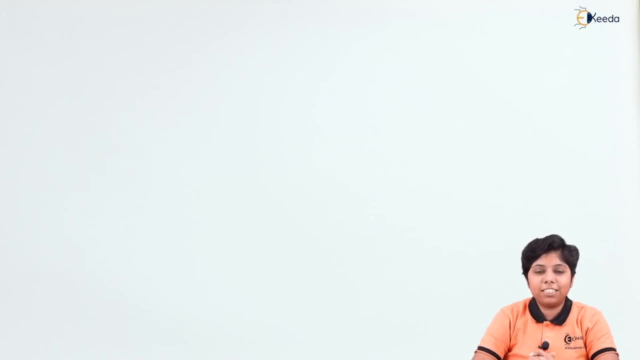 and better stick to this wind, wet and wet die algorithm. the next section: we will talk about deadlock detection now. we will talk about this deadlock detection now. the deadlock detection is a situation that is different from the deadlock prevention in that way that the deadlock is now prevented and now we are in a system we are looking for if there is any deadlock or not. 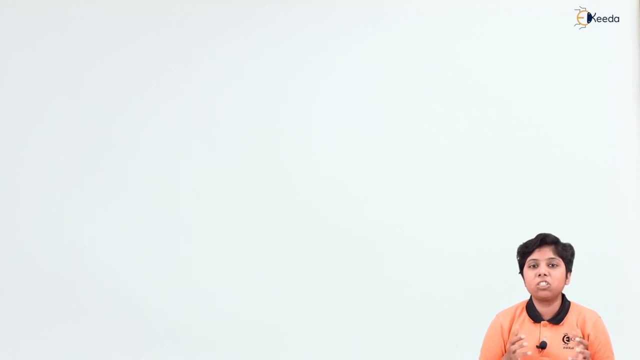 so it is more like the deadlock prevention. but it is not before the system has started that we are not arise in the situation that the lead lock will not occur, but they are in a situation on a system that deadlock can occur and we need to detect that if 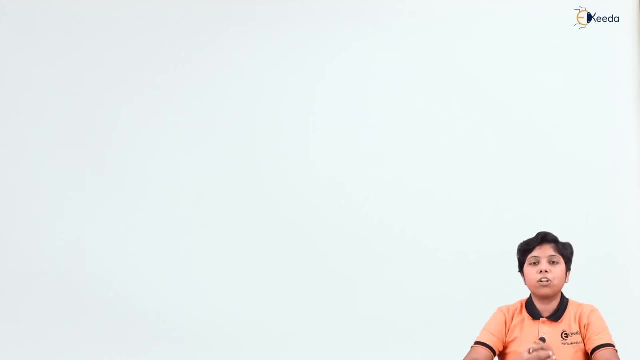 there is any deadlock or not. so for the deadlock detection we need to maintain the information that, whichever the data or the transaction that are locked and data item and is requested for a data item on particularly- we will describe a graph containing all the information about this one- that the request and the lock timeout. 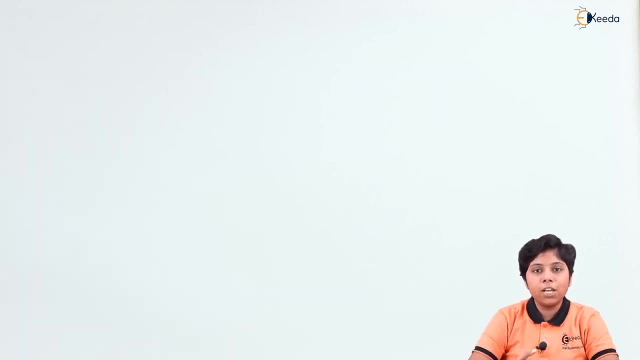 and the deadlocking and finally release the items in a way so that we cannot have any deadlock any further. so the first one for this deadlock detection is an approach for an wet for graph. so this wait for is in directed graph where we can say it is in set of v and e, so the g is the graph. 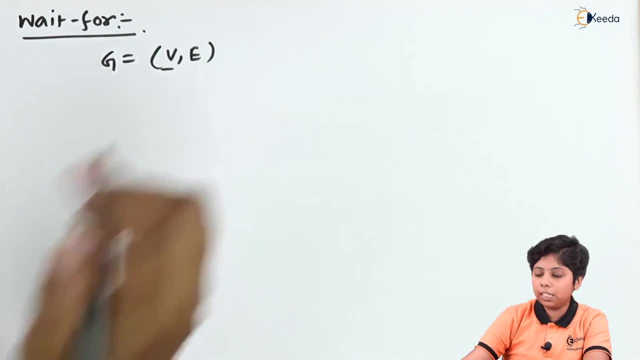 which is a set of v and e, where v is the vertices and e is in directed edge towards this t i g. so when we are having this t i h to t j, that means t i is preceding the transaction t j. so now t i is waiting for an item that is tj is holding to release the item to finish its transaction. 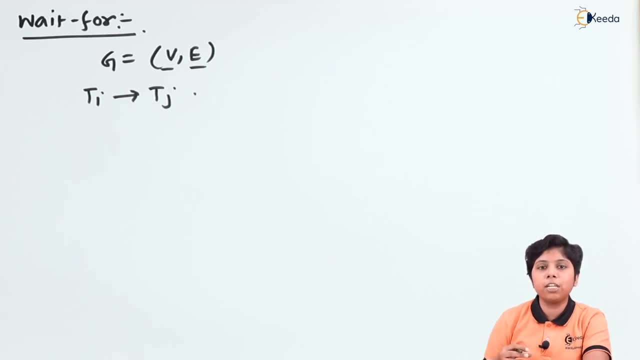 now we will add in this graph each transaction that is waiting for a data item that is hold by another transaction in this one, and if there is any request that has been fulfilled, then we will remove this edge from this graph. and if the graph is containing no cycles, then we can say that the deadlock is not present in the 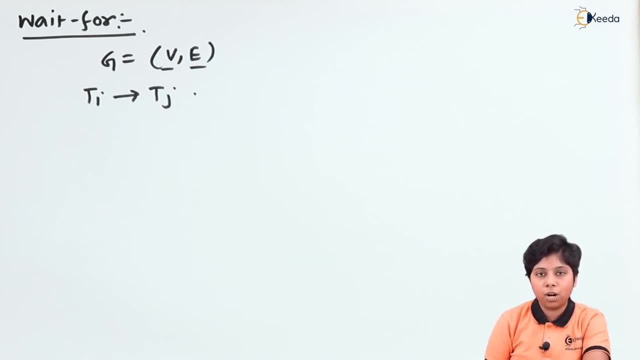 system and if it is present in a cycle for that graph on an wait for then we are saying that the deadlock can occur or occurred in some cases on that system. so now let us first define this wait for graph with an example. say: suppose that first the system introduces the transaction t1, so it 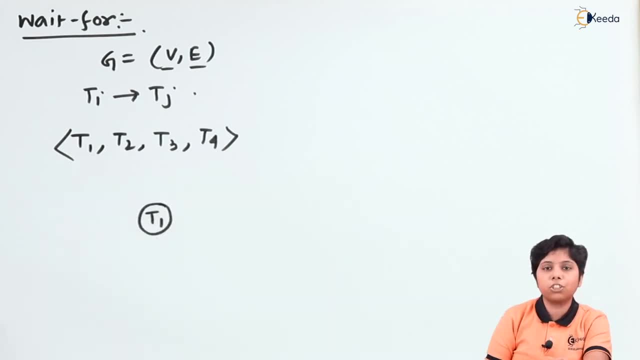 will be introduced in the vertices set on this transaction on the graph. so now t1 is performing its transaction with some of the items that is locked by t1. say suppose t2 is now there, arrive in the system and it requests for some data items to be locked which is now held by this t1. 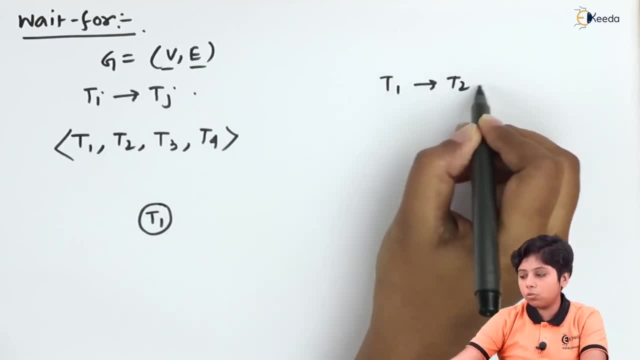 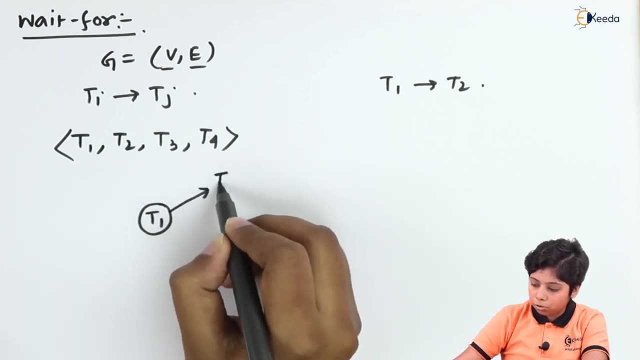 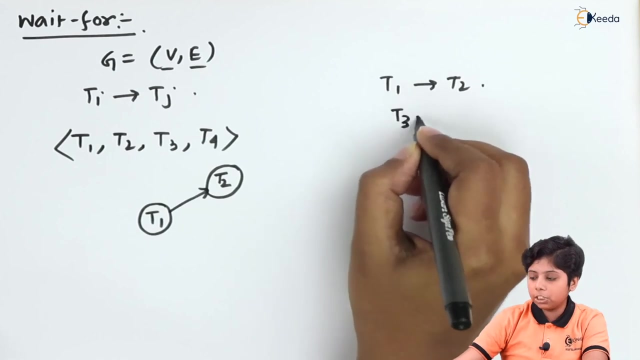 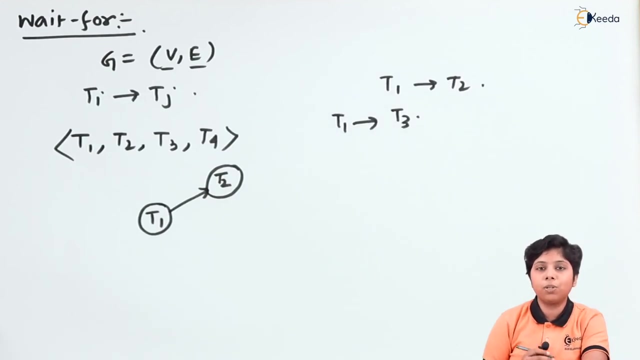 so now t1 to t2, we can say that t2 is waiting for that trade item. so we can add this edge t1 to t2. now we are saying that there arrives another transaction, t3, in such a way that t3 also waits for t1 to finish its execution or t1 to release the item. so now we will add a directed 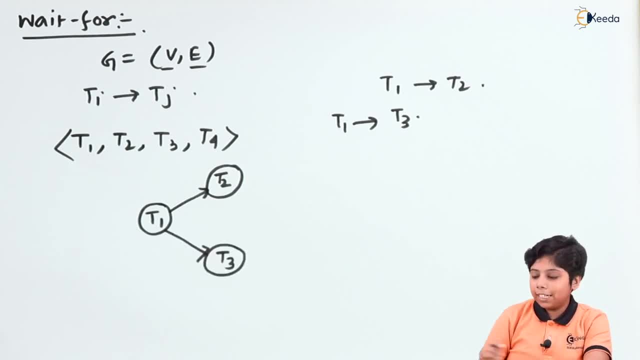 edge towards t1 to t3. now we say that t2 is also waiting for some items that has been released by t1, held by t3, and now it is waiting for the transaction t3. so now we are saying that t2 is this T2 to release the item from T3. So there is a directed edge from T3 to T2.. Now, finally, T4. 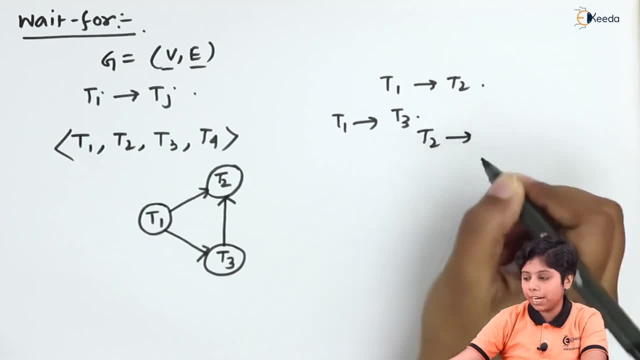 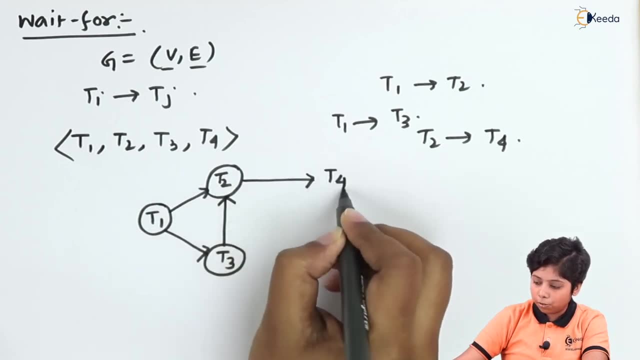 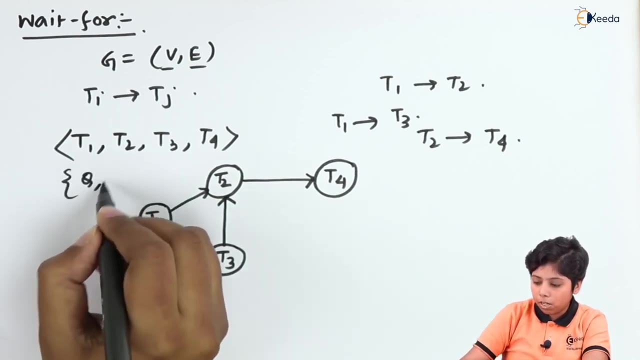 arrives in this situation that it wants for some data item to be released by T2. So now there will be a directed edge from T2 to T4.. So in this here we are having the data item set Q, R and S. So first we are having T1, with the data item locked with Q and R, Now T2. request for R. 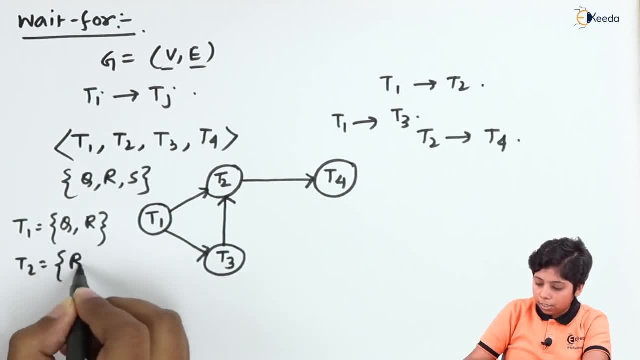 So now T2 is waiting for R. that goes with this directed edge. Now T3 arrives and it wants the data item Q and S. So it is allotted the data item S and now waits for the data item Q and S. So it is allotted the data item S and now waits for the data item Q and S. 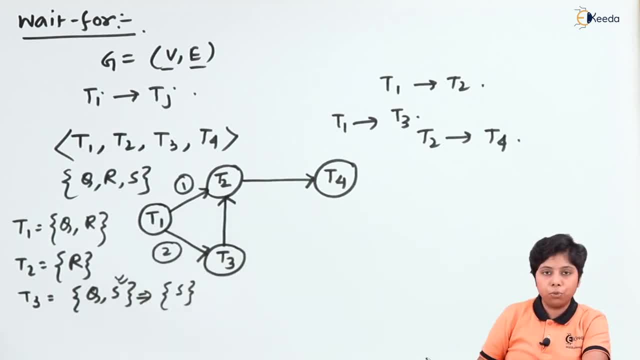 Q. so it is wait for the data item Q. now T2 also waits for the data item S. that is held by T3. so now T2 waits for both R and S and has not given any of this data, so it waits for this T3. and finally T4 arrives with the request for Q and S. 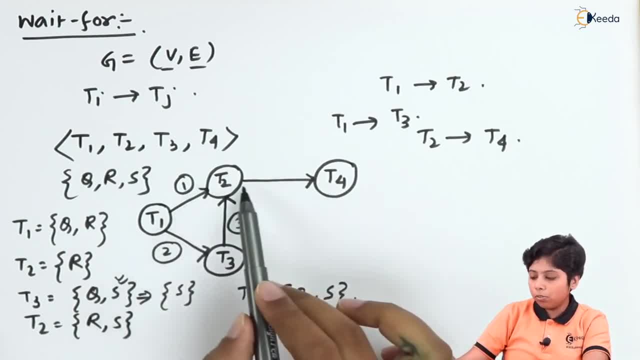 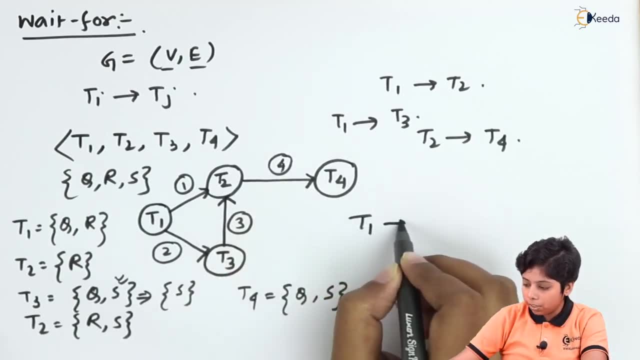 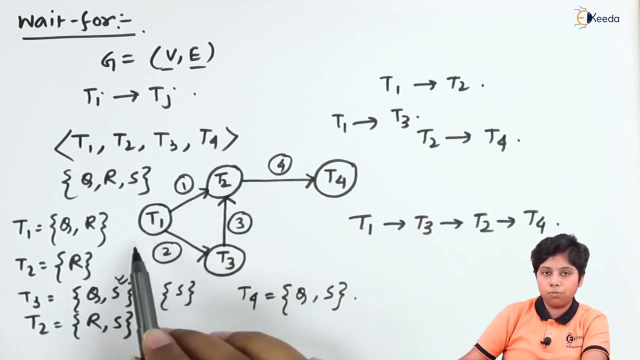 that is now held by this T2. so there is an request H for this one. so now we can say that we are having T1, T3, T2, T4 and no cycle to it, because T1 from the T2 and T3, T3 to T2, but there is no directed H from T2 to T1, which doesn't make a 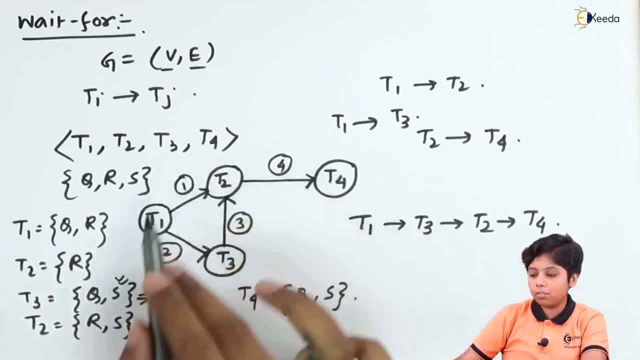 cycle to it, so we can say that the system on this graph is not having a cycle to it, so we can say that the system on this graph is deadlock free, or we cannot detect any deadlock from this graph now if we arrive in other conditions with the other state of data items and also the 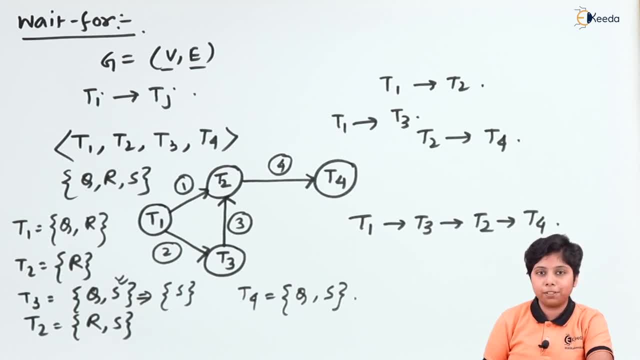 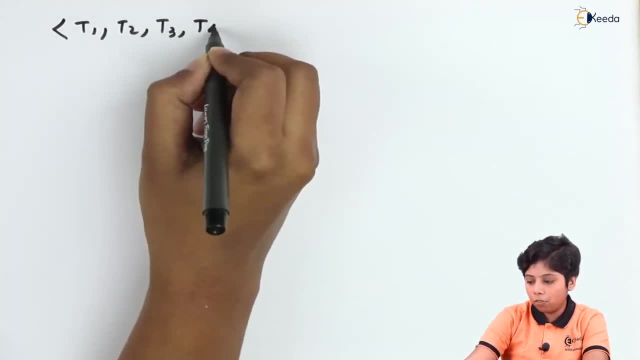 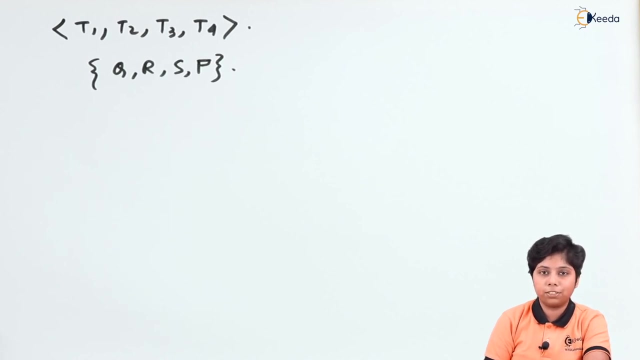 set of transactions. now let us look for another example. now let us constitute with then another T1, T2, T3 and T4 transaction cycles with the data sets Q, R, S and P. so now we are having four data items with four transactions. so first, T1 is 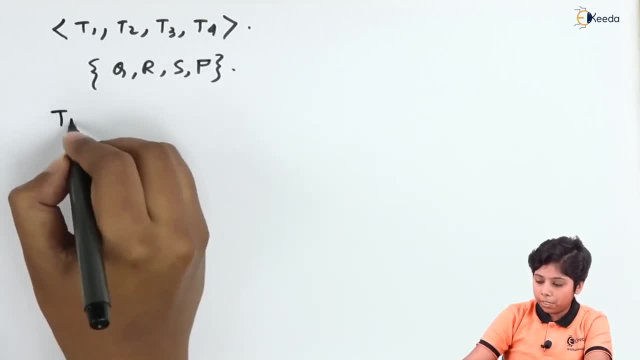 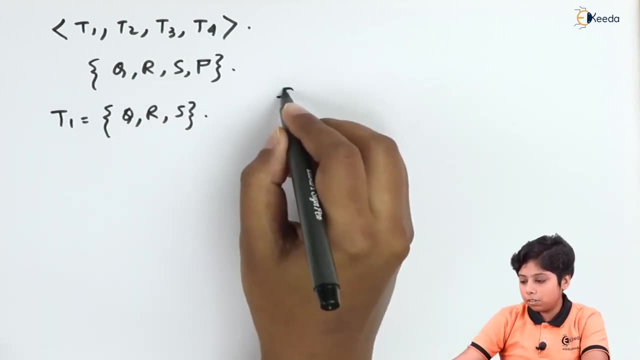 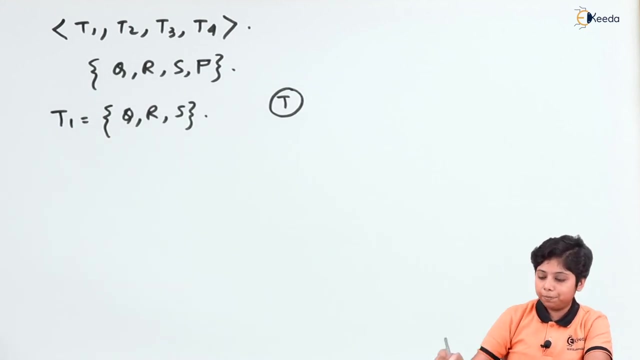 requesting for Q R and S. so it will be given Q R S. so T1 is present in our graph. now T2 arrives with the request of R and S to it. so T2 arrived within request R and S and it is waiting for T1 to release it. so now there will be an H from T1 to T2 after. 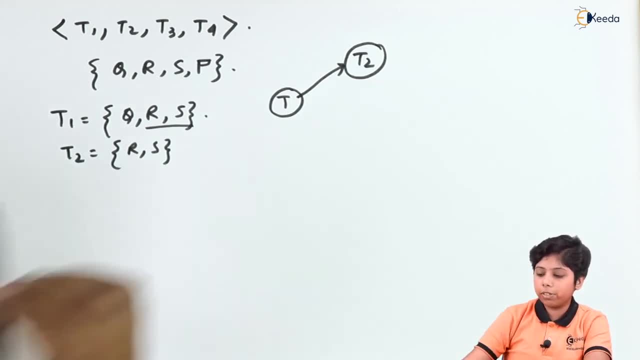 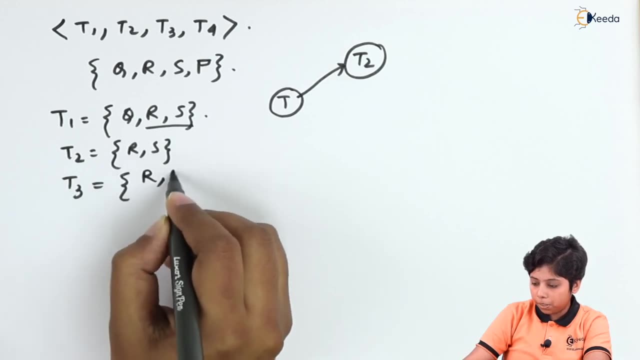 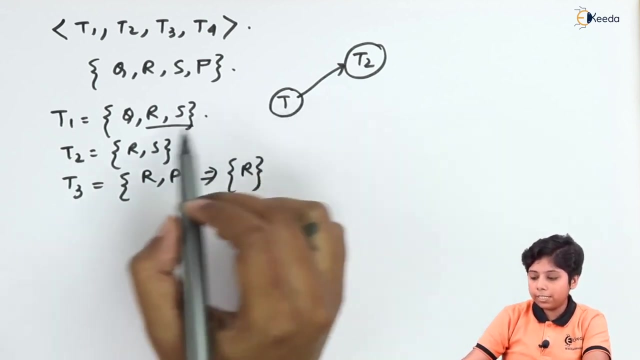 that T3 arrives with an operations, that is request for R and P. so T3 arrives with R and P. from that it will be allocated P. now it is waiting for R, so the R is held by T1. so now there will be an request H from T1 to T3.. Now say there is a release that we can arrive to T2, which we can. 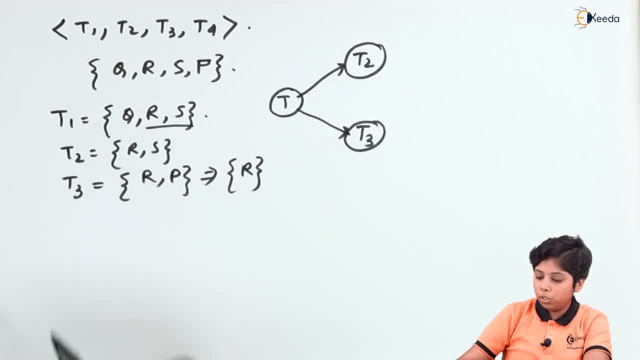 have from this R and S and from this Q. So now T2 goes for the weight of R S P. So we are having P as a request from this T3 which it is holding. So it will concur and request H from T3 to T2.. 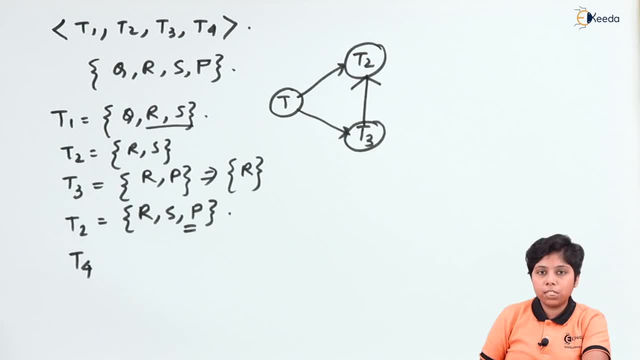 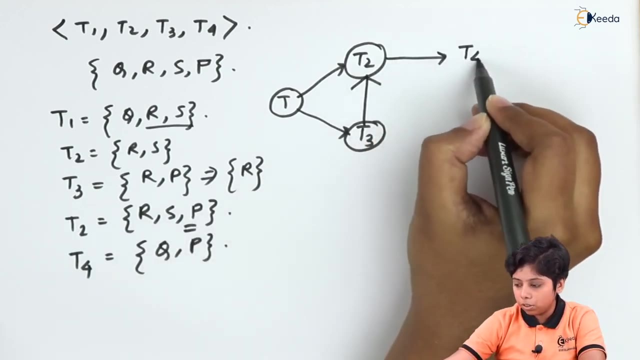 Finally, we can say that T4 is arriving with this result set that it wants Q and P. So now both are the items that is held by T2 and it is waiting for it. So there will be a request H from T2 to T4.. Say suppose: 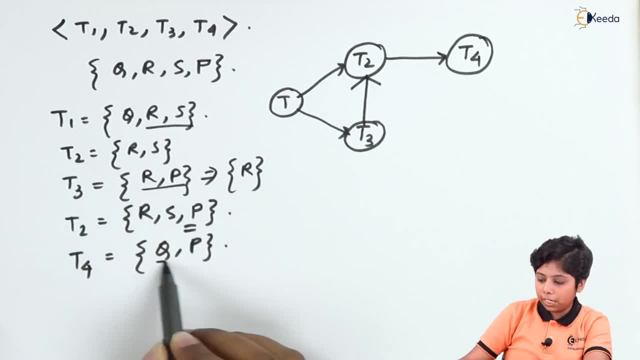 that we have a request H from T2 to T4.. So we are having P as a request from this T3, which it is also waiting for R and P, and here also it is waiting for Q and P. So there will be a request. 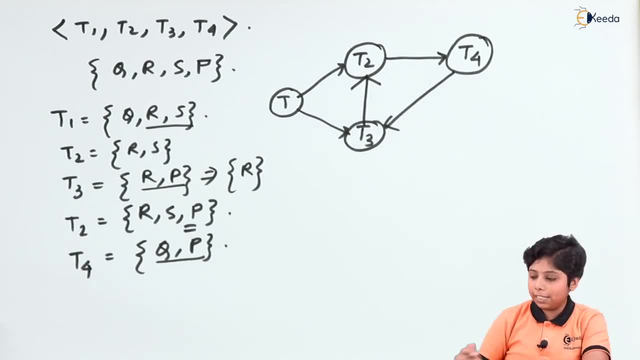 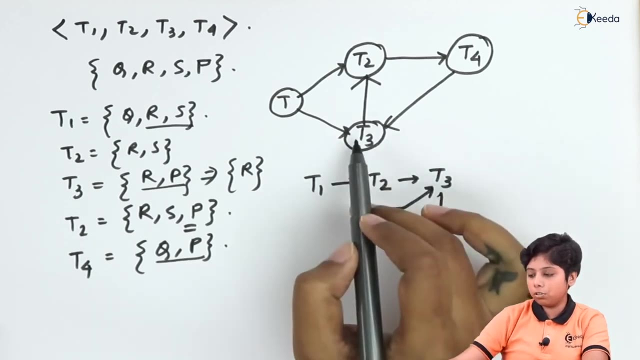 H for T4 to T3. Now we can see that T1 goes to T2, goes to T3, goes to T4. Again, it goes to T3. So there is a cycle for T3, T2 and T4 which we are having in this graph. Now we can say: 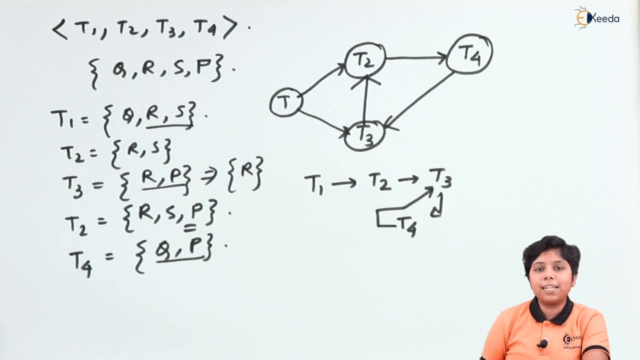 that the deadlock has occurred, So as the deadlock has occurred. so how much the deadlock will affect the transactions? And should we remove all the transactions for our wait for graph or just we remove the transaction that has been affected? So we cannot say that how much. 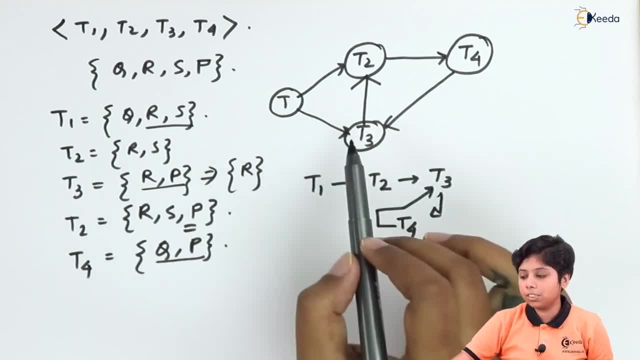 frequently the deadlock will occur. If the transactions are involving in this deadlock or number of more, then we need to perform this wait for graph more frequently To detect the deadlock. And if we are having less number of transactions that we can perform at a time interval to detect this deadlock, Now suppose that we are having this transaction. 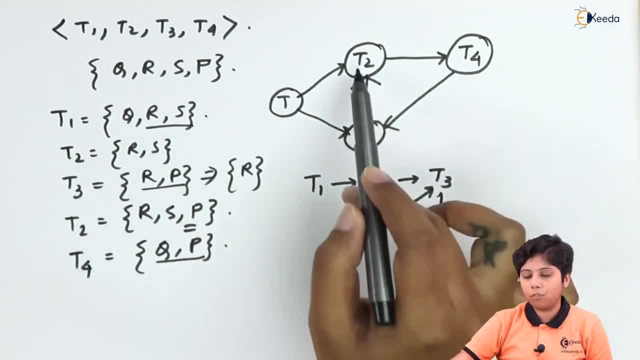 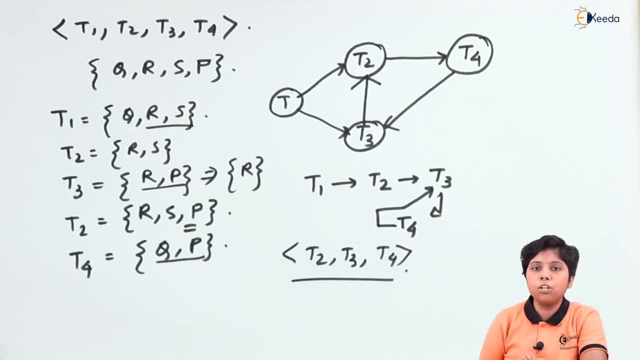 that is involved the deadlock T2, T3 and T4.. So we need to have this T2, T3 and T4 restored or rolled back their execution so that we can have the wait for graph without any cycle. But T1 remains there. 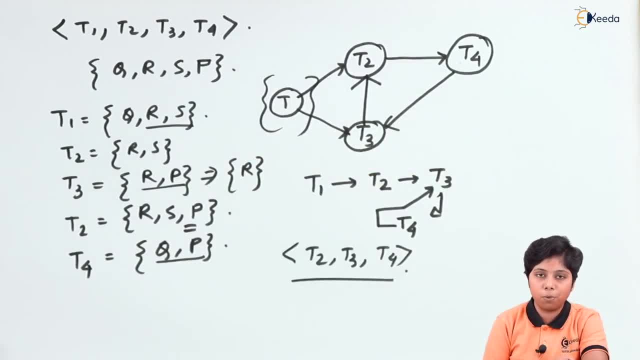 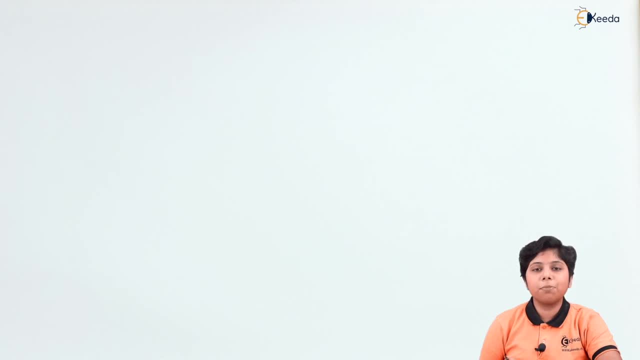 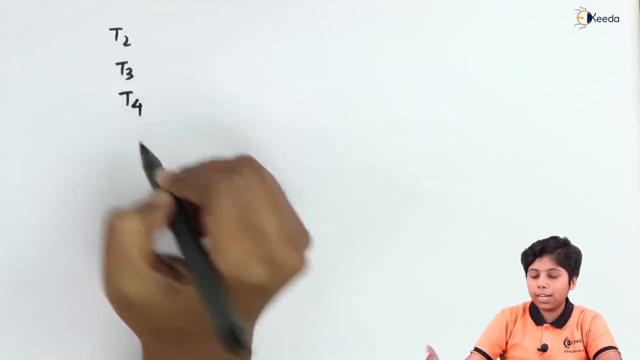 In this graph because it doesn't constitute to the deadlock problem. Now let us move to the deadlock recovery. So first one is the selection of victim from the deadlock detection algorithm, As we can see that there is T2, T3 and T4 that are the 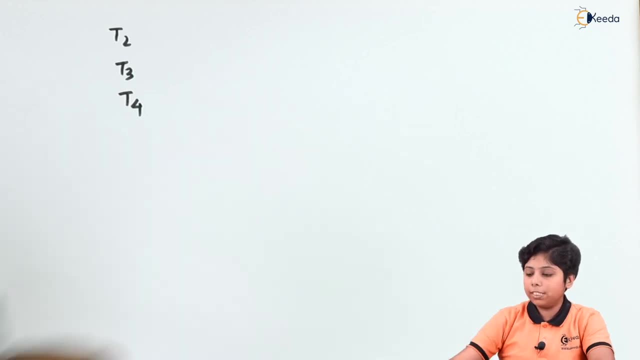 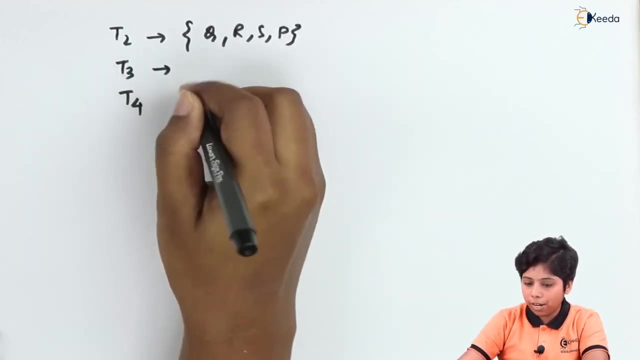 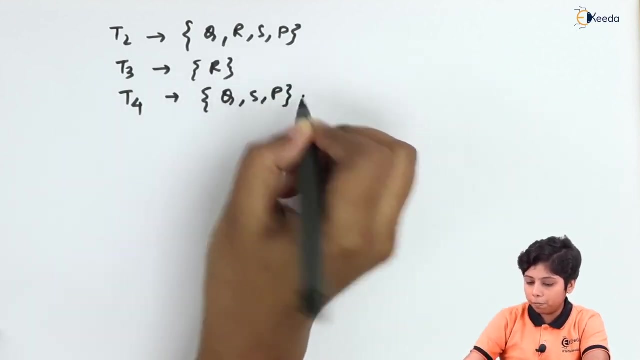 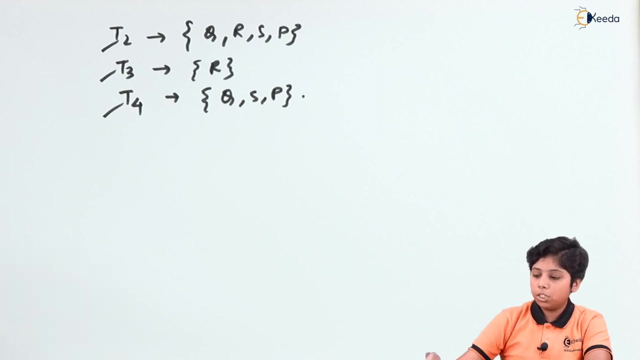 transactions that were involved into the deadlock. While T2 is requesting for QRSP, T3 were requesting for QRSP. So now we can say that T2, T3 and T4- that is which is the selection on this- victims. So we can say that T2 is the most dangerous victim in this deadlock because it requires 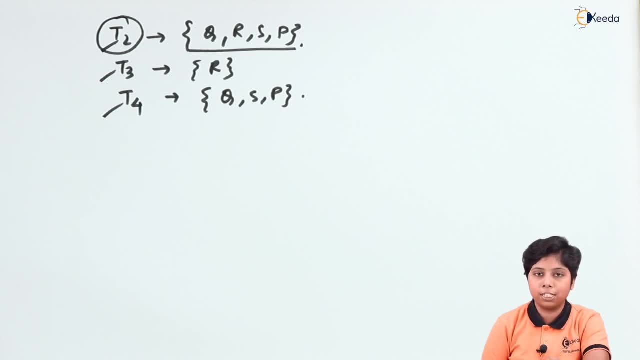 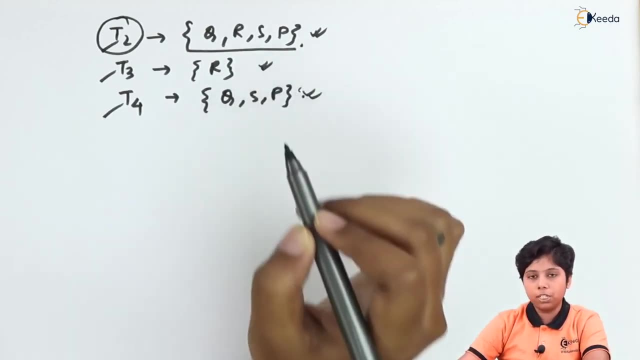 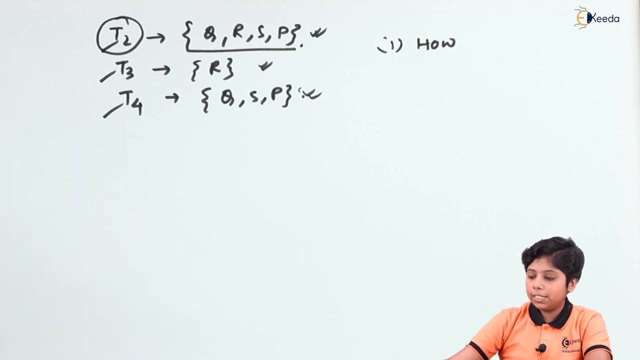 four of these variables, which is helped by some other transactions. So now we need to recover this T2 first, after that this T4, after this T3.. So the first question is how much dangerous on these transactions are. The second one is by what frequency they are occurring. this transactions on deadlock If it is on a less. 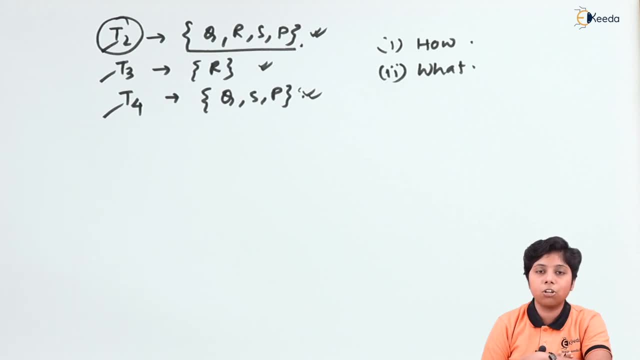 number, then we need to produce the numbers on the transactions on a rollback. Second, the recovery techniques required two of this process. The first one is the rollback, The second one is the starvation. When we are talking about rollback, then we have two types of 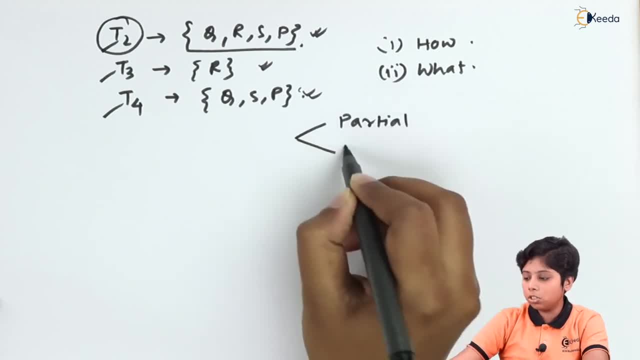 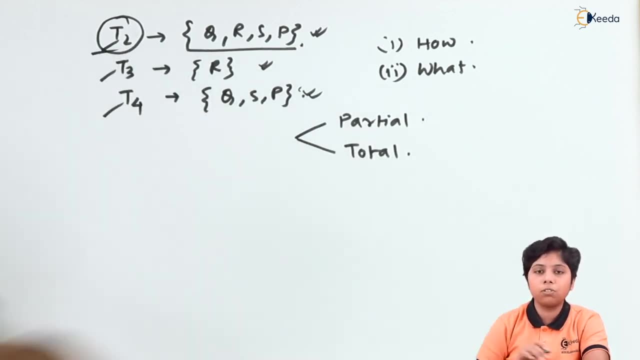 rollback. One is the partial rollback and another is the total rollback. The total rollback or an abortion is the system is terminated for that particular transaction and has routed within refresh and all the transaction has been performed or not. Now the partial rollback is if there is a need for a particular transaction after a period of time. That means the wait. 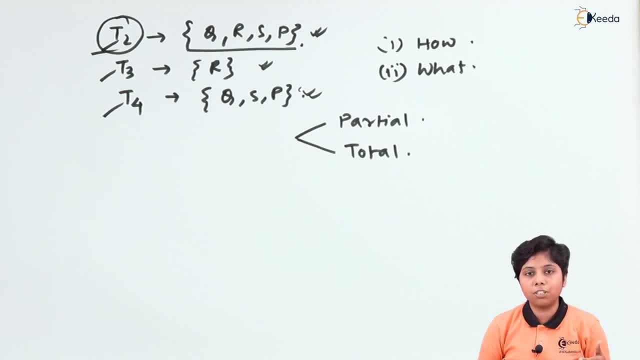 for time graph is frequently checking the deadlock for the detection. If it is detected for the deadlock, then it will go for an partial rollback to the situation or till the statement on the transaction which does not involve the deadlock situation. Now, if it is from the beginning, then we will go for an total rollback. Other than that, we